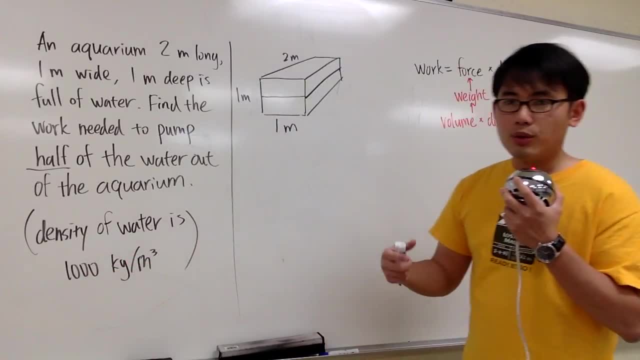 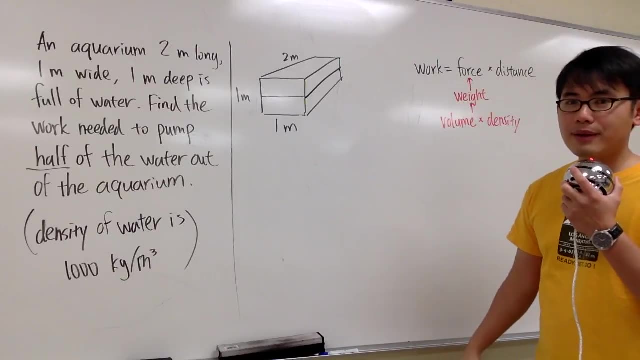 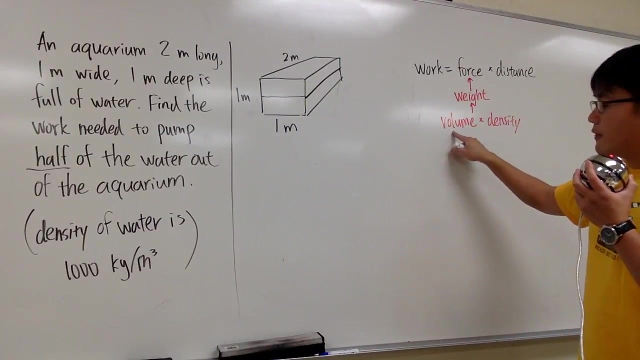 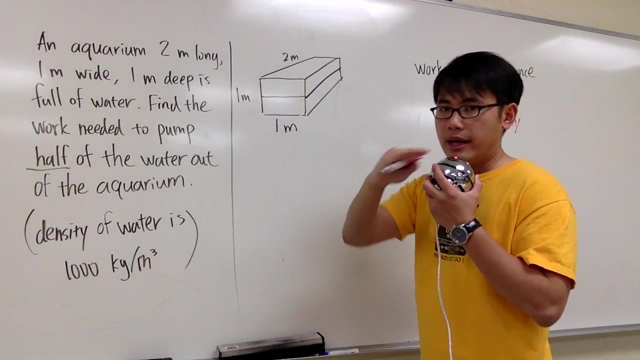 kilogram per cubic meter. And then we also have to multiply by 9.8 for the gravity, If we are using feet, and we just need to multiply by 62.5.. By this situation we'll focus on 1000 and then the 9.8.. So for the volume, this is how we are going to do it And we'll just focus on the top half. And the deal is: let's draw a rectangle and then just cut a horizontal slice first, And in this case we get a perfectly 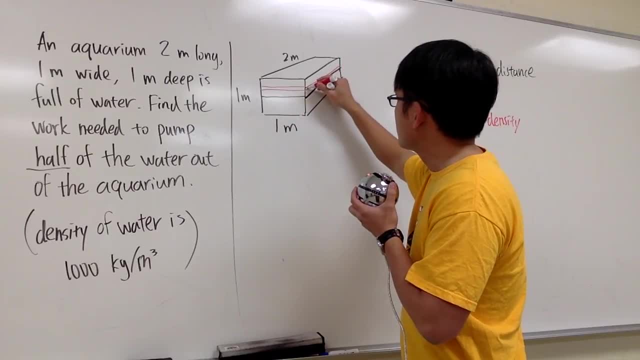 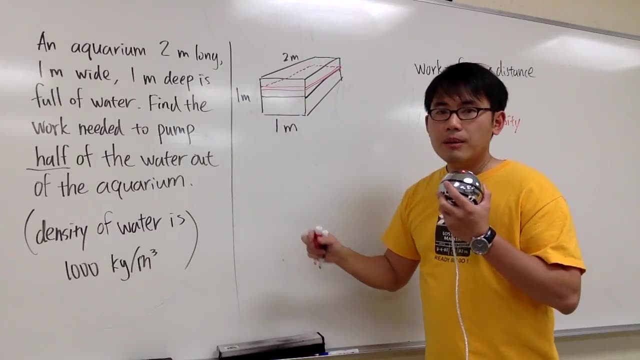 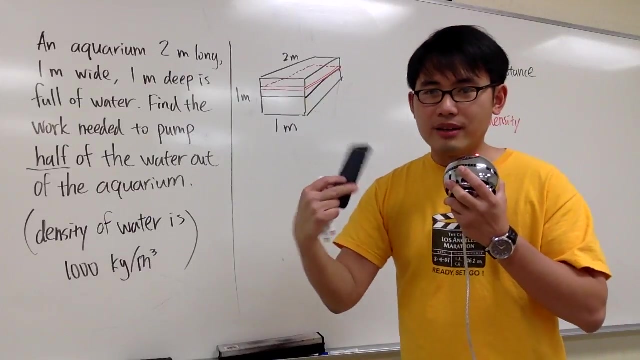 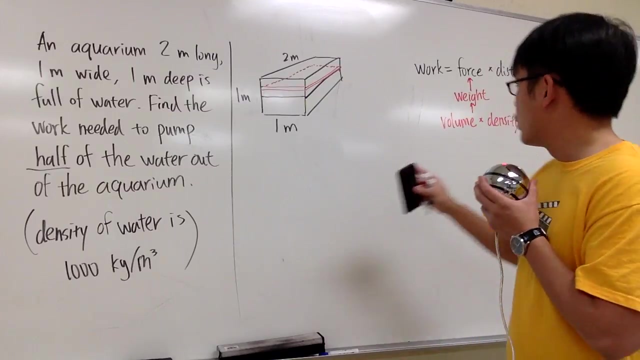 rectangular slice, because the Korean is rectangular in the first place. So you can see, this is pretty much the picture that I'm drawing. It's not the best picture, But then what's the shape of this slice that we just draw? It looks like a phone, right, Because it's rectangular. So, as you can see this right here, it's pretty much the slice that we're talking about, And the goal is we will have to write an expression for the volume of this slice of 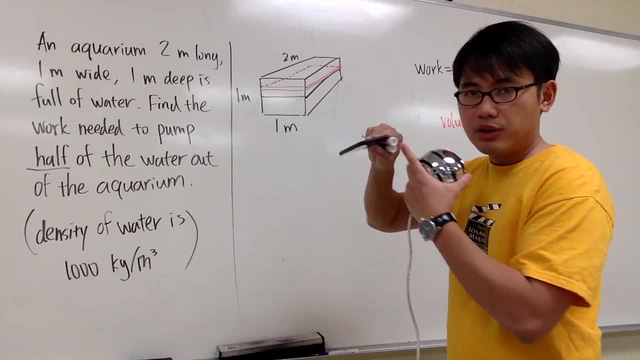 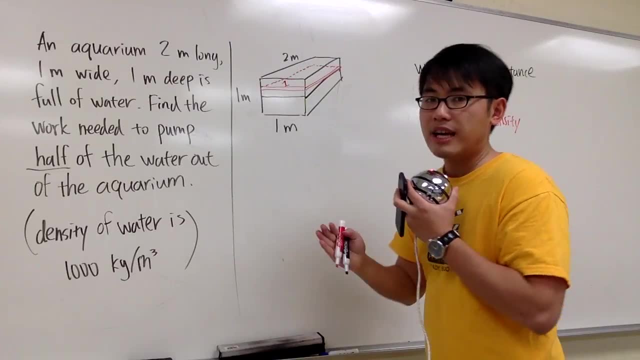 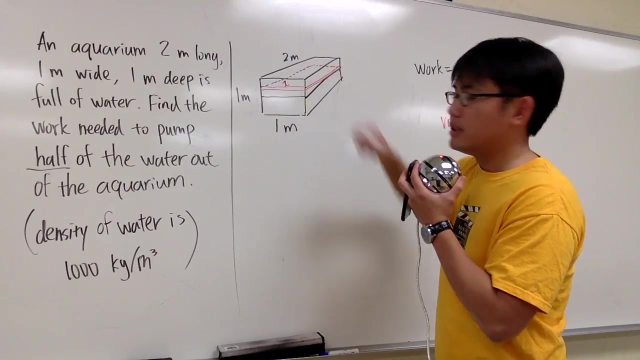 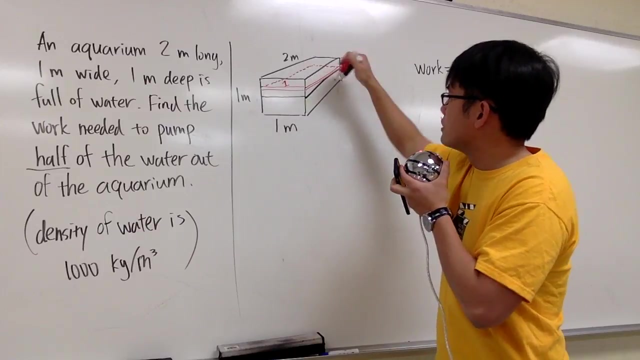 the water. So first, do we know what's this measurement? So, the front part right here, This part, we know it's equal to one meter, And that's really nice, because it never change, right, It's always one meter, it never changes. How about, how long is this? Well, it's this long, right, It's this long, which is two meters long. So this right here is two. And how about the thickness? This is just a small. 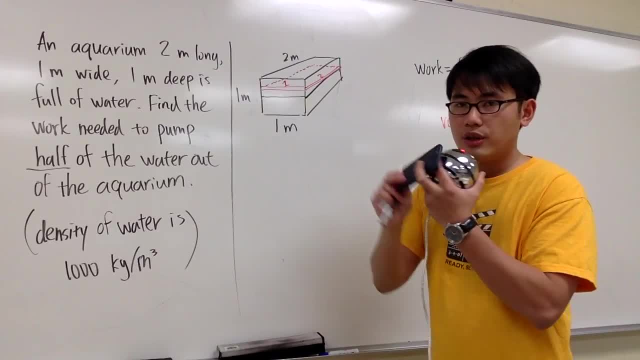 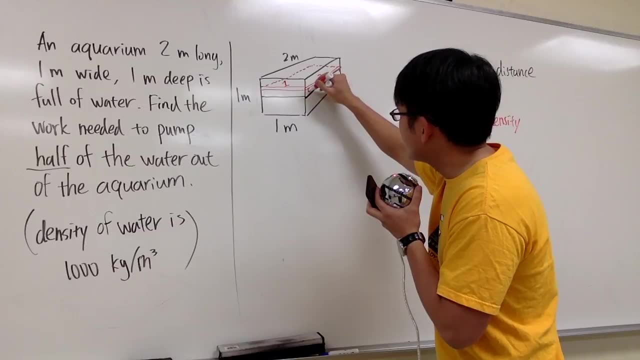 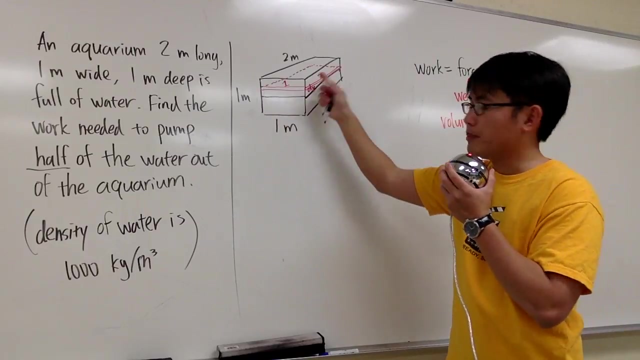 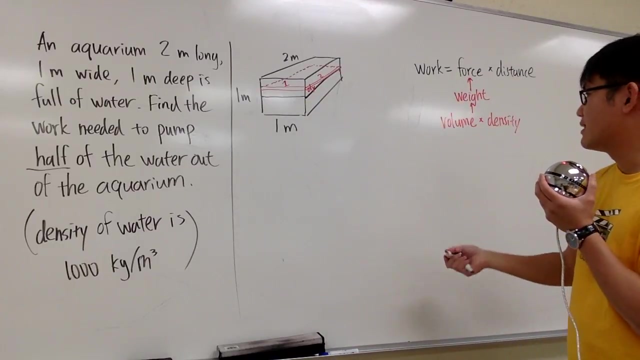 change amount in the y-axis, because it's a vertical change, right. Just a small change amount in the y-axis. I will just label this dy. So just look at this and then call that to be dy. And now we are ready to write the expression for its volume. A volume for this rectangular box is just one times two times dy. That's it right. Length times, width times, height. So I'll just put this down for the volume: one times two times dy. 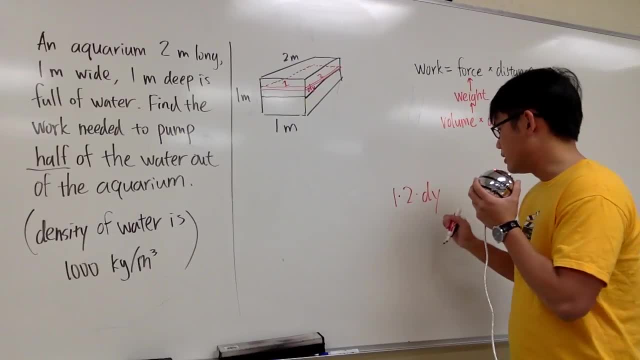 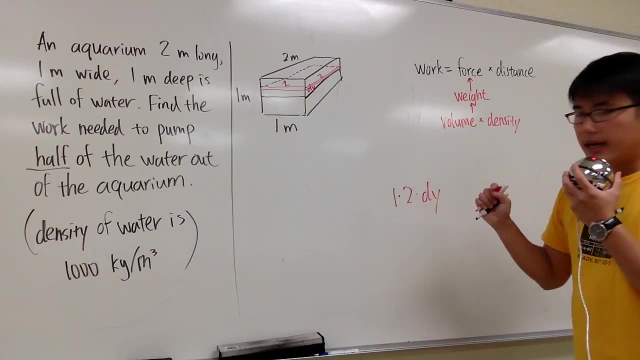 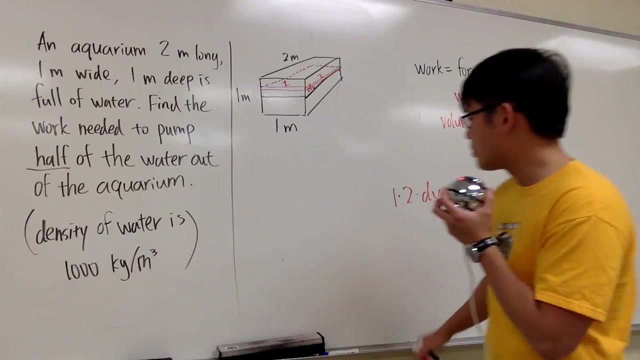 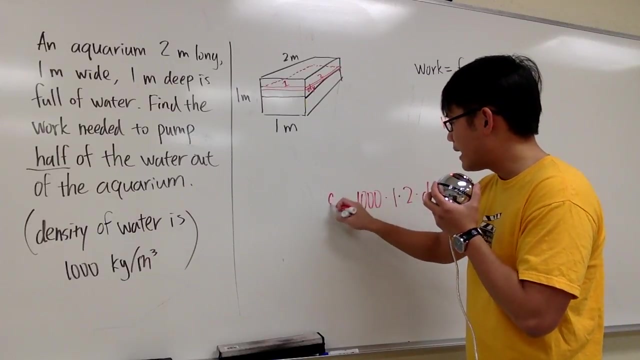 And then in the meantime I'll build up my integral, So I'm using dy and then I'll put the dy all the way at the end. So that takes care of the volume of this slice. And then the next thing is the density And the density of the business. the density business is once again the things I mentioned. We just need to multiply by 1000.. Okay, for the water density and that's a mass density. And we also have to multiply by 9.8 for the gravity, because one meter- All right, that takes care of the volume. 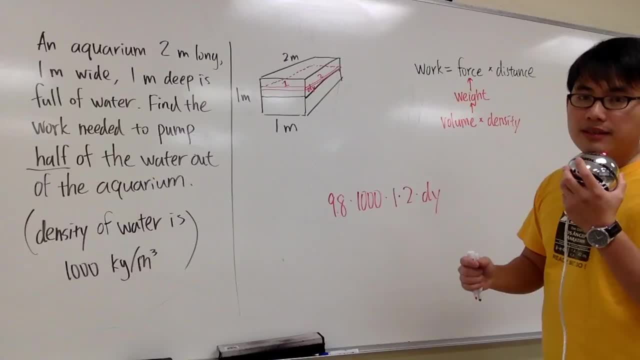 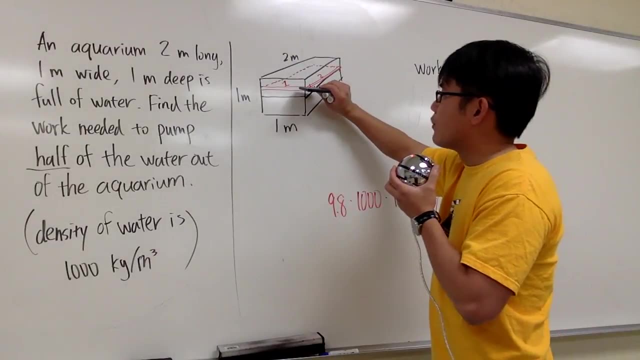 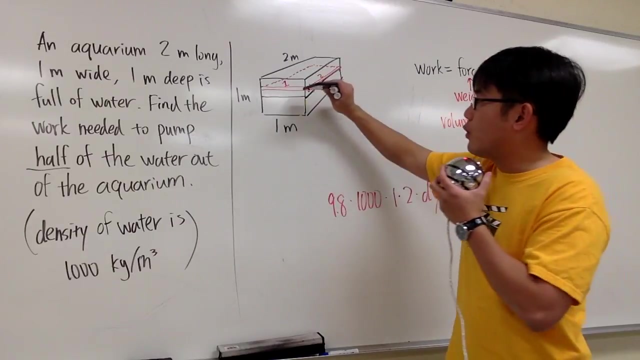 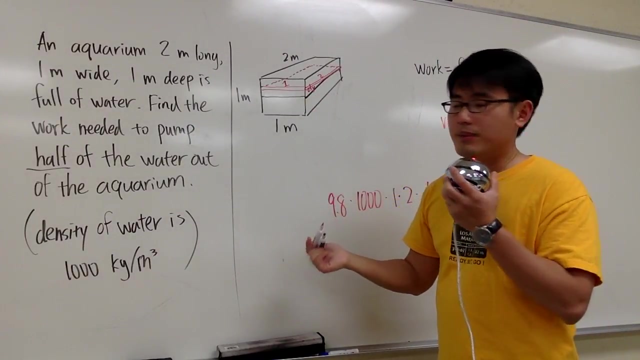 And now we have to figure out distance. And for the distance, it's usually based on our labeling most of the time, And the idea is: this is a slice of water that we are talking about. How far do I have to travel from here up to the top in order to pump out this amount of water, this slice of water based on labeling? And in this case it doesn't really matter how you label it, because it doesn't have a lot of restriction, Because 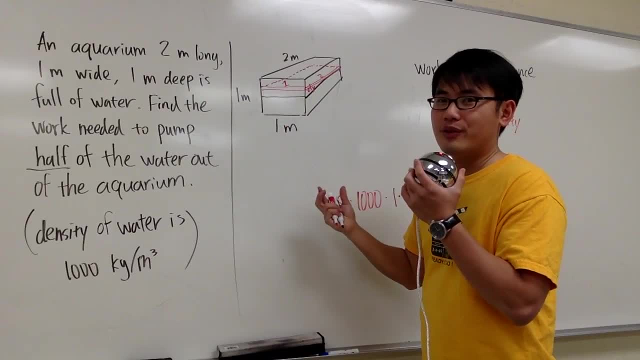 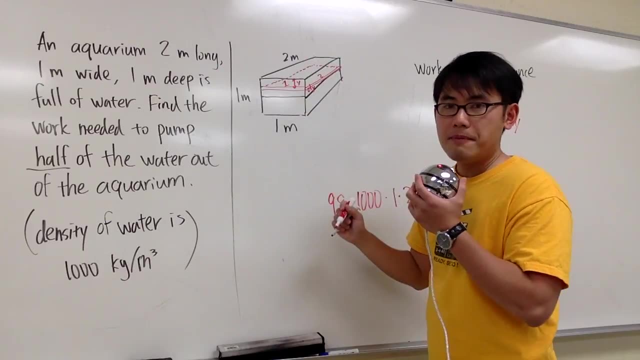 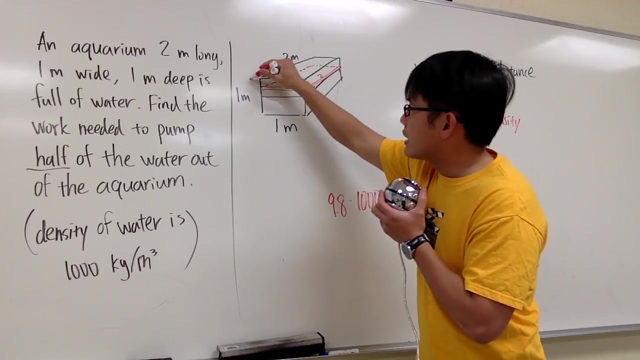 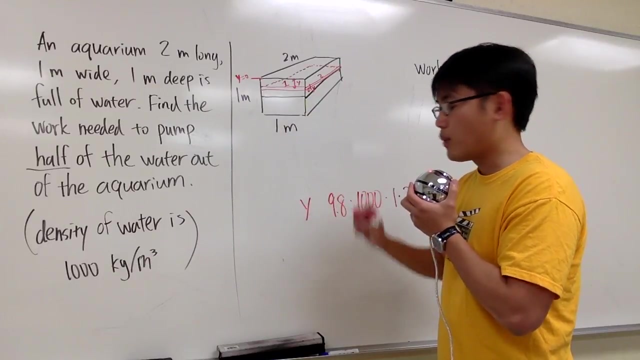 this is constant, that's also constant. So it's pretty straightforward. If you would like, I'll show you. we can label this as y, from this distance as y. you can do like that And let me put that down right here. If you label this amount of distance is y, where you take this is y is equal to zero. That will be the distance, And I'll just put down: we multiply by y for the distance And I'll put on this right here in black. actually, This much, 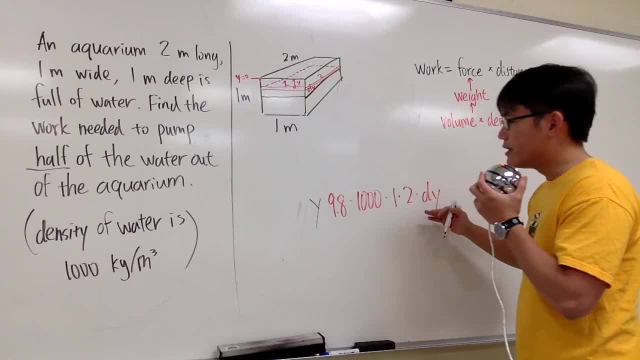 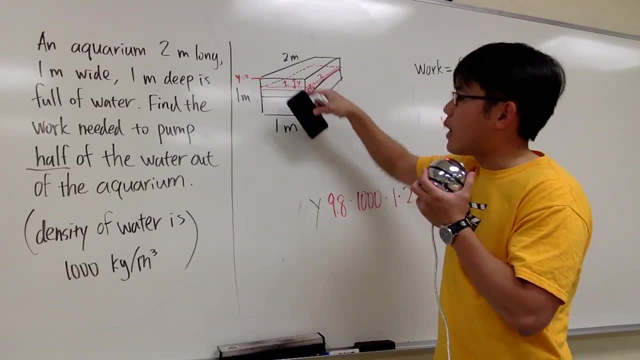 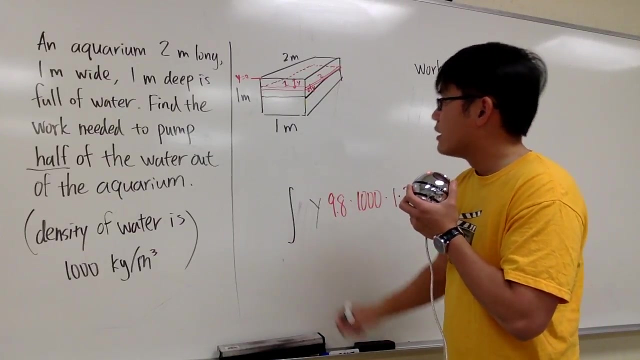 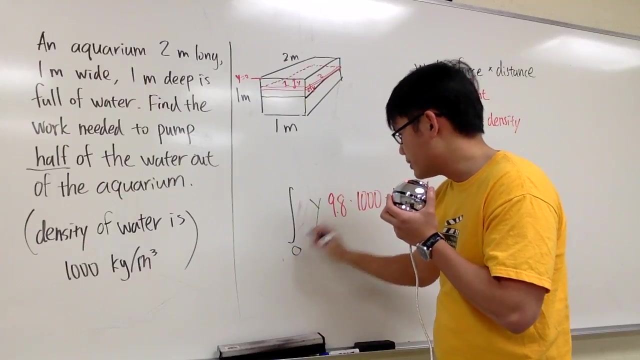 right here is y. This right here represents the work that we need in order to pump about this slice of water. the distance that we travel is just y, And now we have to do a lot of this and that's the integration part We integrate. the first y value is technically zero, right, because that's the surface. we pick that to be zero at the first place. So we pick this to be zero, and then we just want to go halfway, So this right here is halfway. 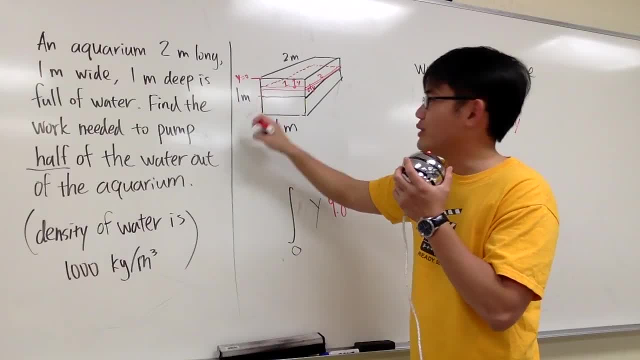 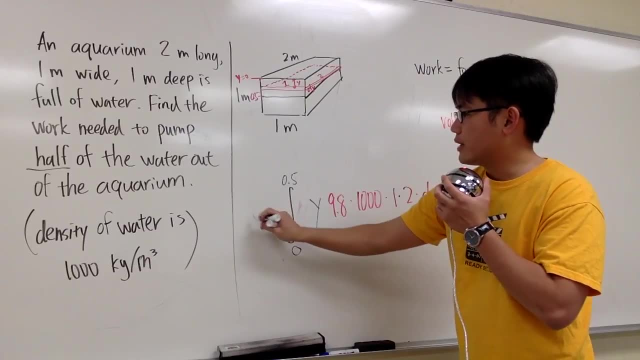 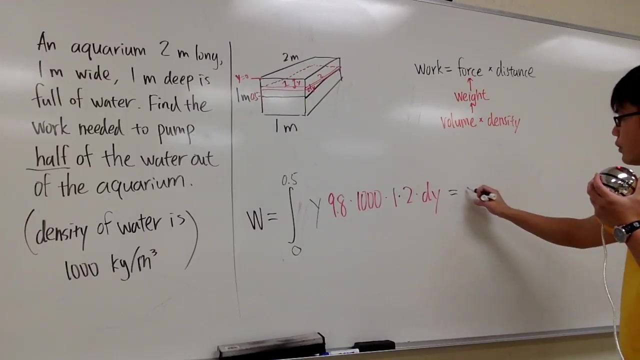 half of what? half weight of one meter, which is 0.5 for the y. so you'll be just going from 0 to 0.5 and this right here will give you the work. okay. and if you compute this integral, this right here will give you 24, 50 and this is in the si unit. so we use jewel. 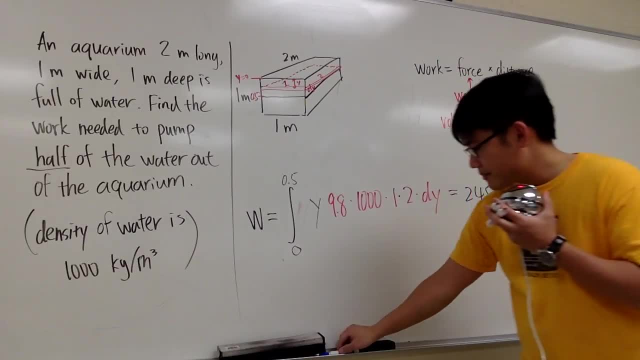 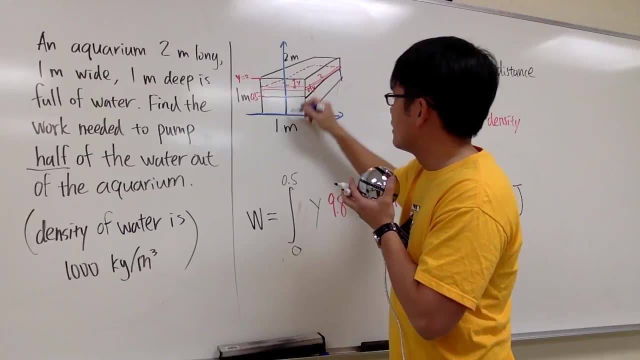 if you would like, let me just mention this briefly. if you put the reference frame down here, okay, if you put a reference frame down here, so this is more like right in the middle and things like that, and you can call this is x, this is y, and 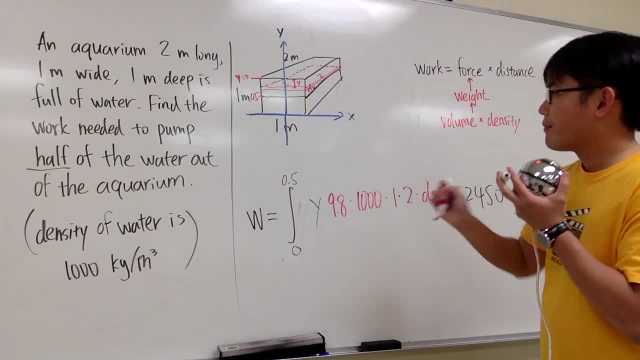 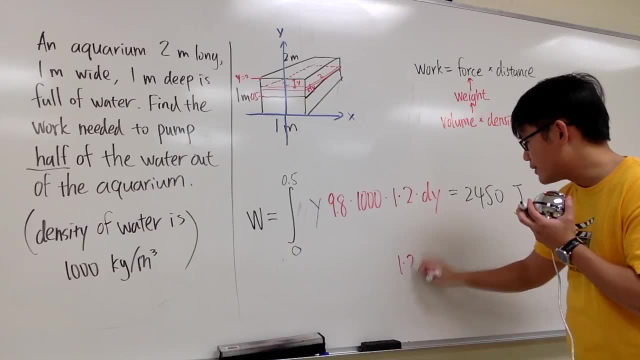 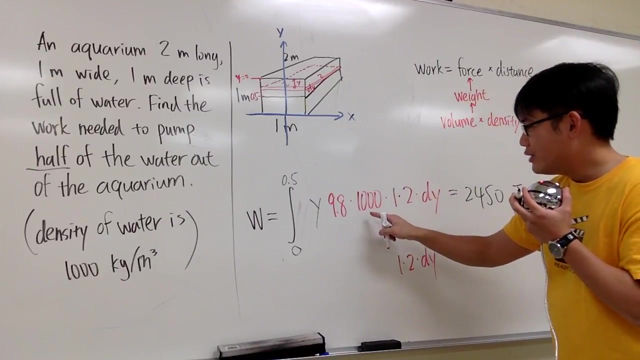 you can set up the integral this way: the volume, the red part, will stay the same. i will still have the uh, one point, one times two times d y for the volume of this box, small box slice of the water. and then you multiply by one thousand water density, mass density of the water, and then 9.8 for the. 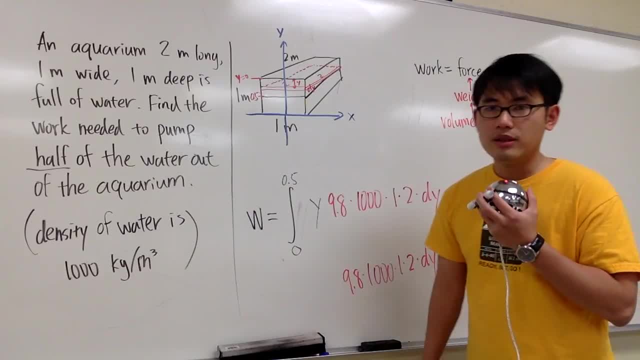 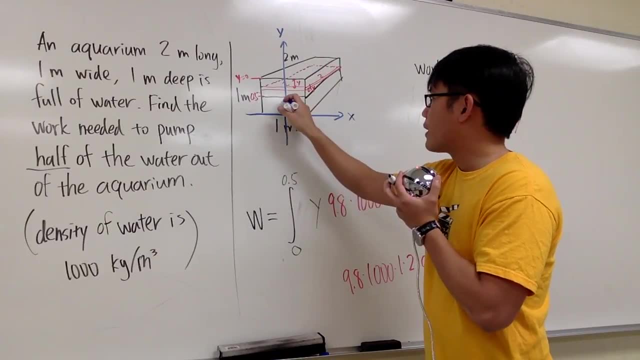 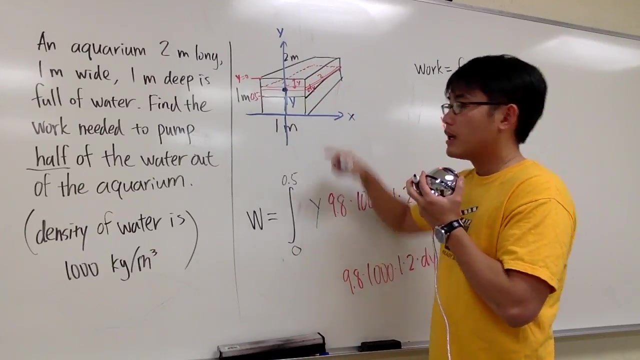 gravity. but in this case, what's the distance that we have to multiply? i'm looking at the blue part. okay, based on this reference frame from here to here, we'll actually actually look at it from here to here. this is the y distance. this slice it's y distance, y distance above the x-axis. so this much. 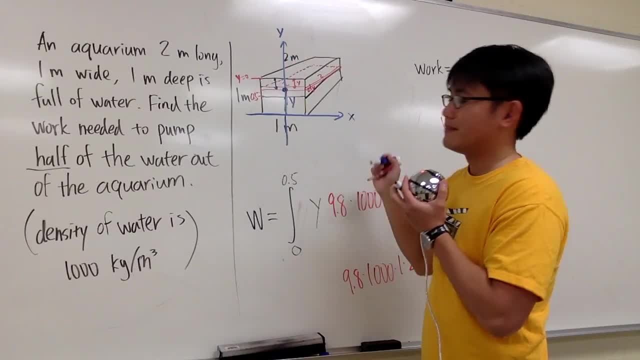 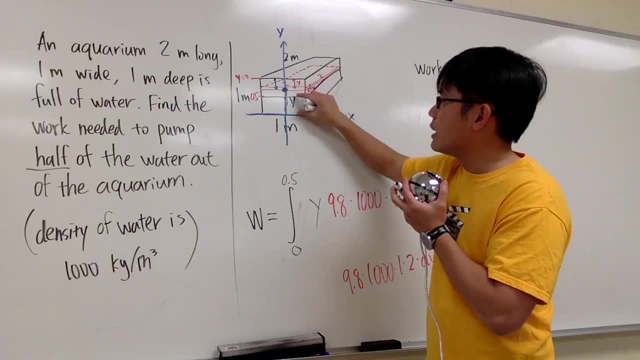 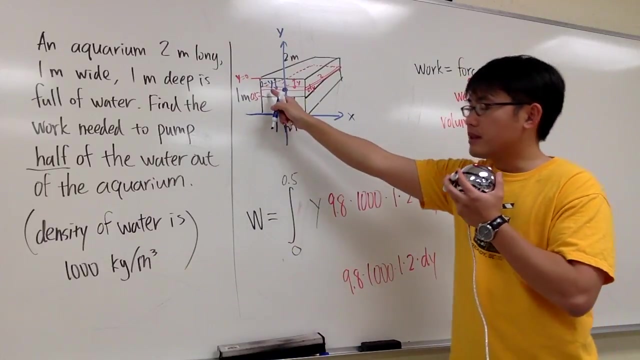 is y and that will give us. this will be what the whole thing is equal to one. this little part right here will be just whole thing, which is one minus this much, which is y, 1 minus y for this right here, and that will be the distance that we have to use, based on that label. 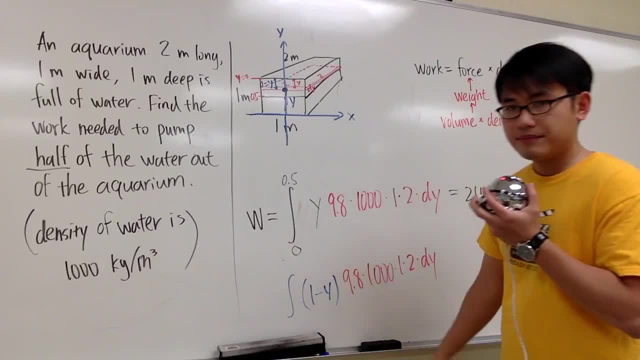 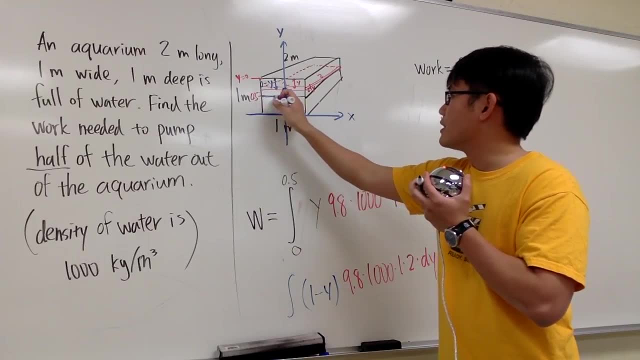 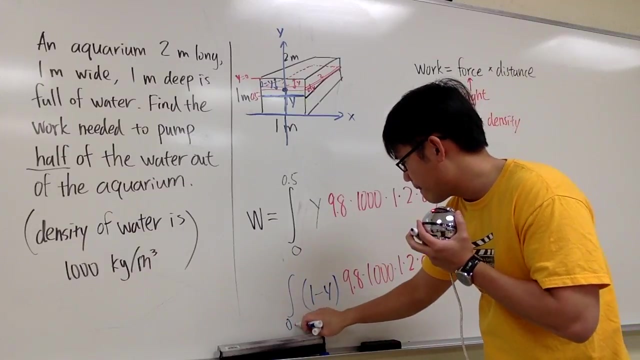 1 minus y. how about the integration? well, based on this, the first slice of water happens right here, because we just want to go halfway and this will give us: y is equal to 0.5, right, this right here is: y is equal to 0.5. and then the last one is going to be: 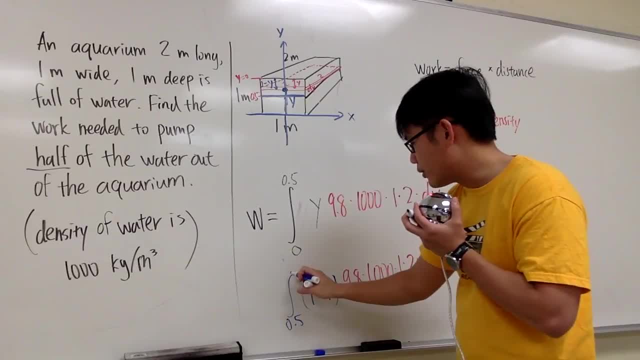 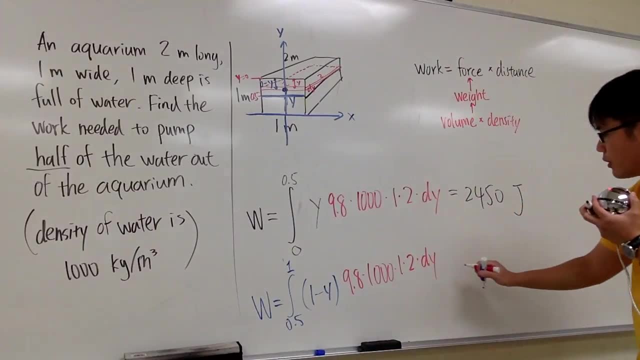 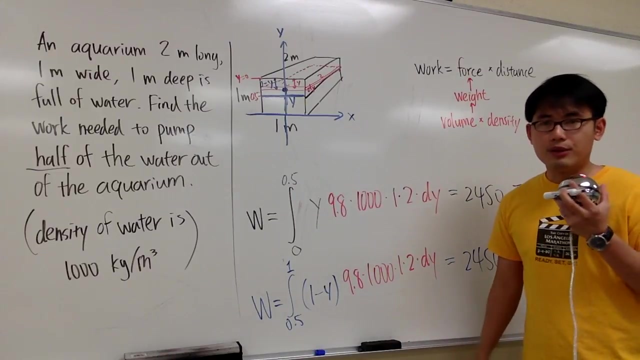 up here and, based on that labeling, this is going from 0.5 to 1, and this will also give you the work. if you compute this integral, the answer to this is also going to be 2450. depends on whichever label that you like. that's it.